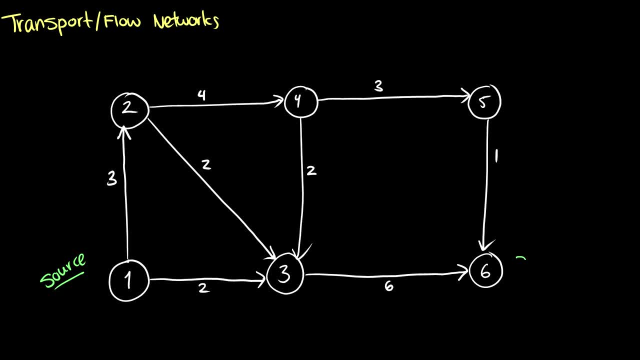 The second main component is the sink. So the sink is the opposite of the source. It has an out degree of zero and its in degree is non-negative, so everything ends up at the sink. So this would be the very end of our pipeline. 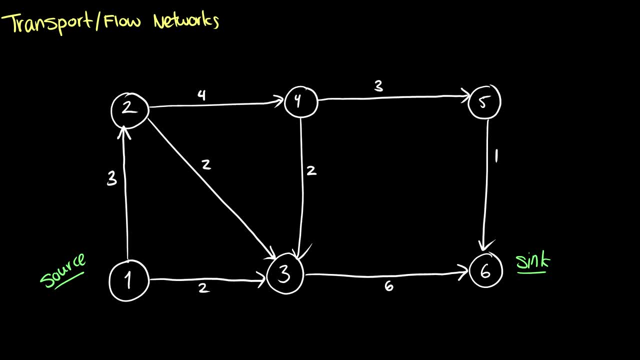 So these are the two main components. The third one is our end. So these are our directed edges. They have a head and a tail And they each have something called a capacity. So this is how much of whatever we're putting through can be handled by that edge. 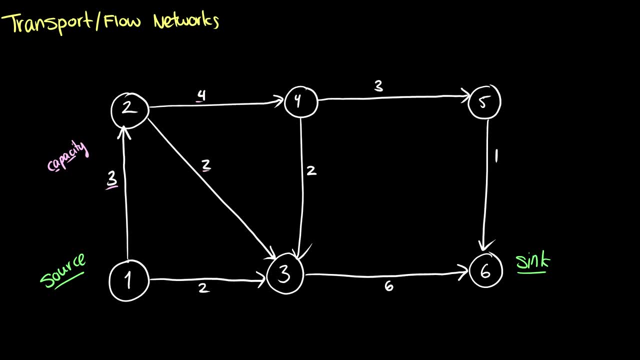 So let's say we have some water in node one and we have, say, four units of water, Then we can only put three up into node two here and the remaining one has to go to three Because we have four units. we have to get through. 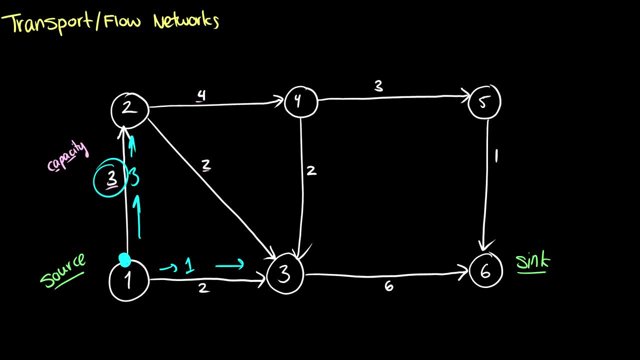 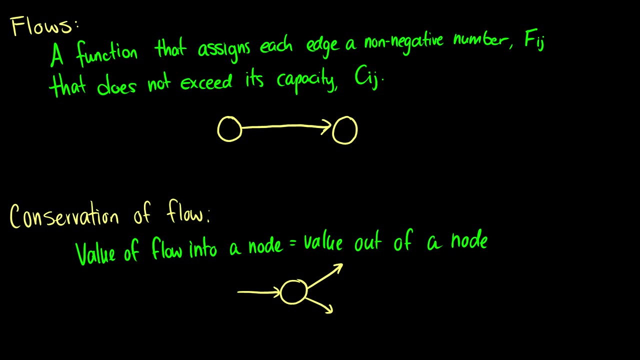 and this one edge here can't hold all of our water, so we have to distribute it to two other edges. So this is a transport network. So what is a flow? Well, a flow is essentially a function that assigns each edge a non-negative number. 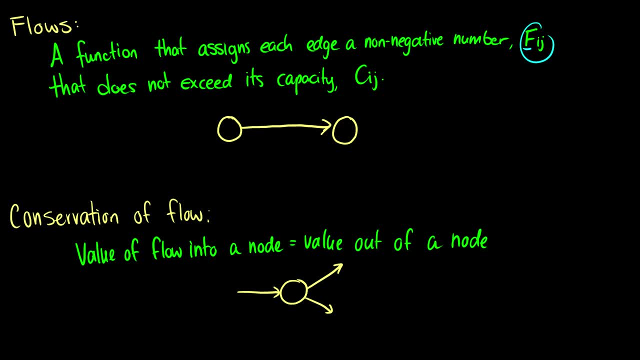 We'll call this Fij for flow and it doesn't exceed the capacity which is Cij. So C for capacity, F for flow. Now remember what I said before is we can have say a three here. 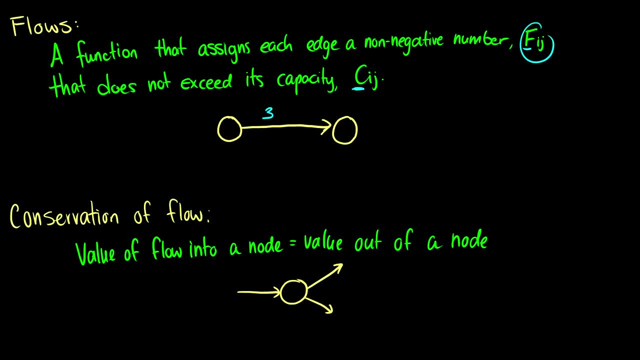 So we can say, okay, this pipe is wide enough for three units of water to get through. So this is our Cij And we can say how much flow is going through. So in this case, maybe we only have two units of water that we have to push through our pipes. 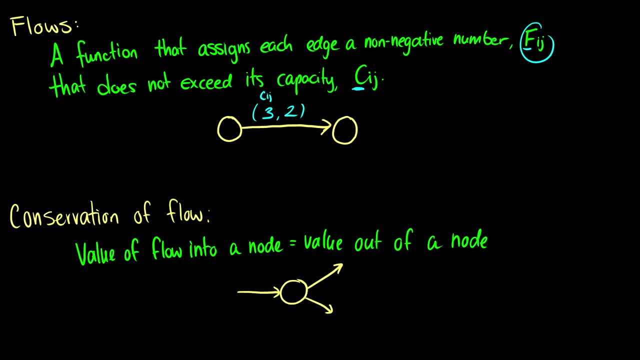 So we can label this edge as as three. two, which means it has a capacity of three, but its flow is only two. So this is what we mean when we say flow. So we can have a whole graph of these pairs with capacities and flows. 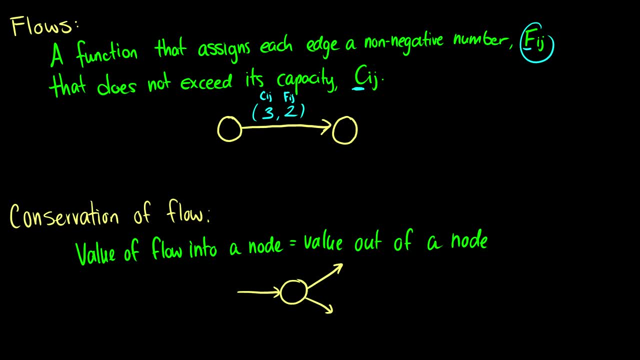 and we can see where all the water is going to. So we have this other principle called the conservation of flow. Now, what this says is that if you have five units going into a node, you should have five units going out of a node. 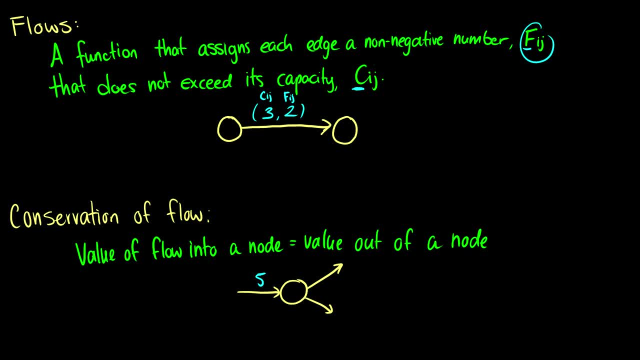 So, for instance, let's say we have five going in, then we should have, say, a three and two or a four and one, or a zero and five. But there shouldn't be more going into a node than it can release. 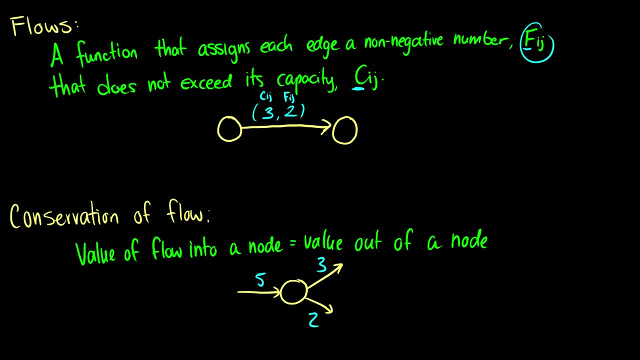 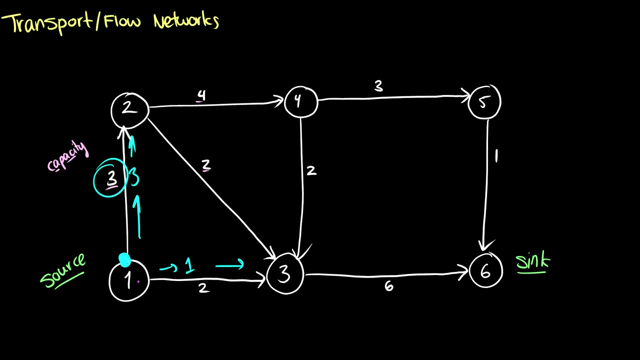 because otherwise we get this blockage and that's really bad for the flow and mathematically not allowed. So what is a nice result of this conservation of flow? Well, that means that if we start a flow at our source, it should be the same amount as the sink. 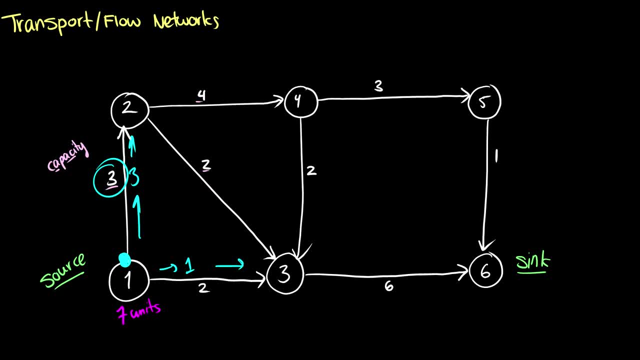 So if we have seven units in our source, we should have seven units in our sink after it travels through. Now, of course, our capacities here are three and two, so there's no way we could get seven out of our source to begin with. 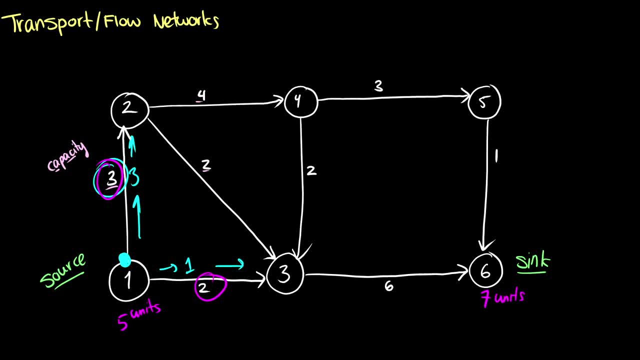 so the most we could get is five here, which means that our sink should have five units at the end, if possible. Okay, So now that we know about our definitions here, the main idea we should talk about maximum flows, Okay. 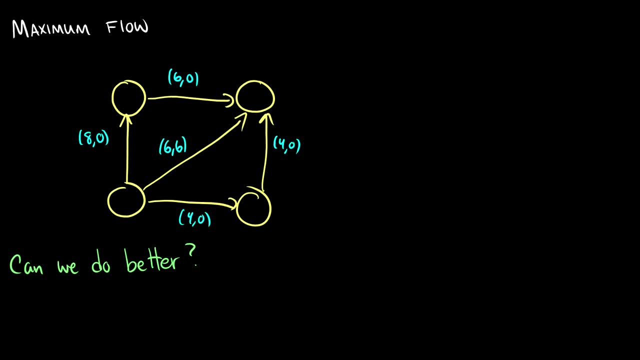 So this is the main problem here. We have a bunch of pipes and we want to get the most water through our pipes as possible. So here I have this little diagraph here. Remember, our ordered pairs are going to have its capacity and then its flow. 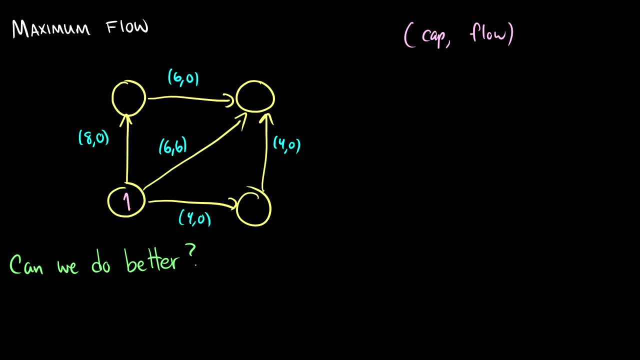 So we have a source node- we'll call one- and a sink node- we'll call four, and we'll just label these two and three And we see, from one to four it has a capacity of six and the whole flow is six. 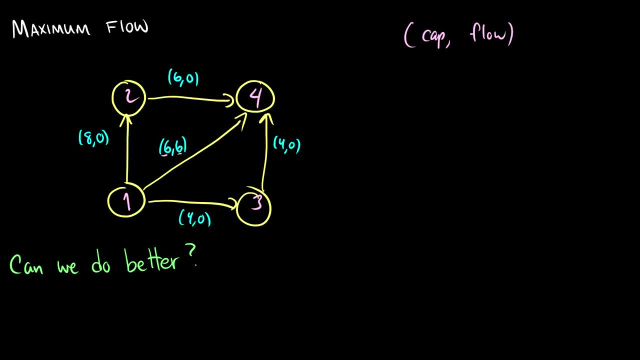 So we're getting six units, from one to four. Here's the question: Can we do better, Can we make this push out even more water, and what's the maximum amount of water we can push through this network? Well, this one's pretty easy to see, because I put these numbers out. 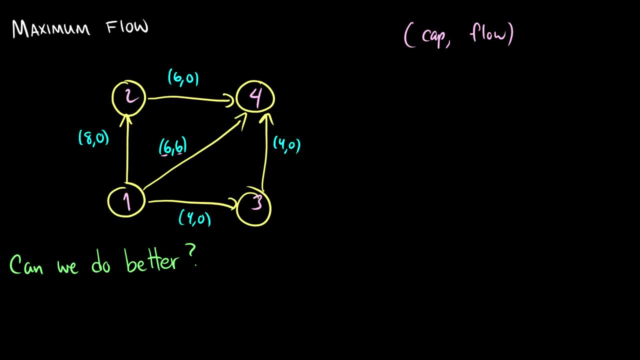 but we can see that there's four units. Four units we can push from one to three and four units we can push from three to four. So we can have a whole total of four going from our source to our sink. And if we go from one to two we could push eight. 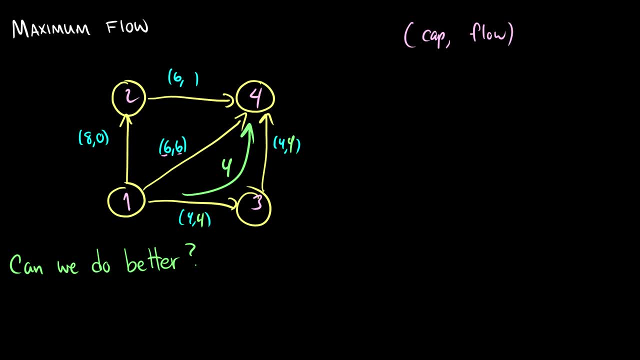 but at this two to four we can only fit six. So we should probably maximize this six and say, okay, well, we can only get six to two and six from two to four, so let's just put six in there. So now, 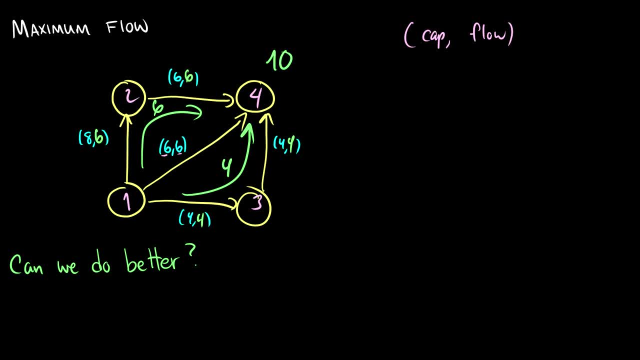 we have six going through that direction. So the best we can do here is getting ten from our source to ten in our sink. So this original path with just six was kind of bad. but we can do better. We could do ten. So that is the problem here. 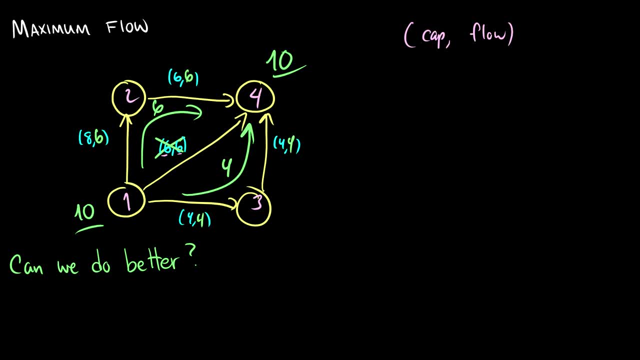 How, taking a graph with more than four nodes and more paths, can we get the maximum flow possible? Well, like all of graph theory, there are algorithms. So this is the Edmunds-Karp algorithm that I'll be talking about today. 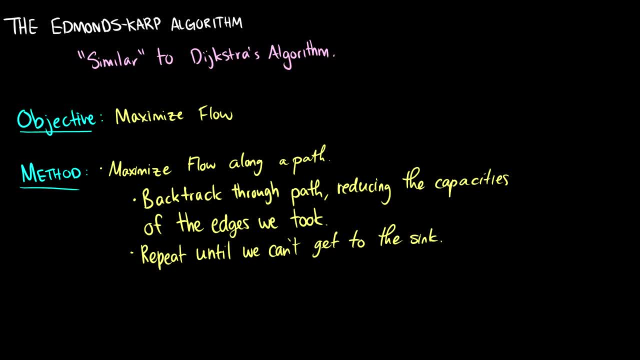 It is similar to Dijkstra's algorithm in a sense. Dijkstra's algorithm was meant to minimize the amount of distance between all of the nodes in a tree, And in this one we want to maximize the amount of flow we can get out of a directed graph. 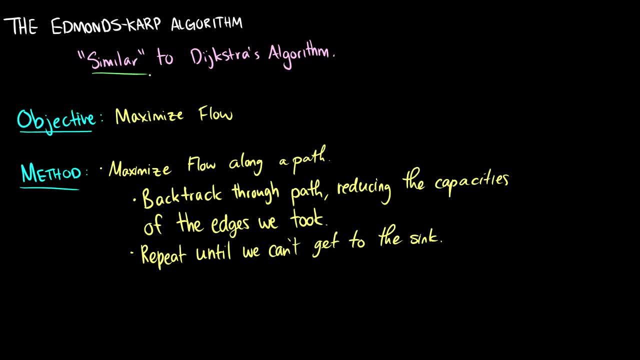 So when I say similar really, I mean not really. So it's not really similar, But if you've seen the Dijkstra's algorithm video, the labeling and the method we use here is going to seem much, much simpler. So I'd suggest checking that out. 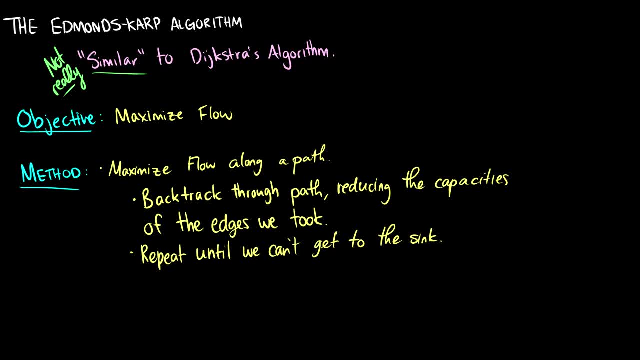 But I'll still go through at a nice pace for this one. So what's the method? Well, our objective is to maximize flow, So our method should maximize flow somehow. Okay, so we're going to maximize flow along a path, So we're going to use up a bunch of our nodes. 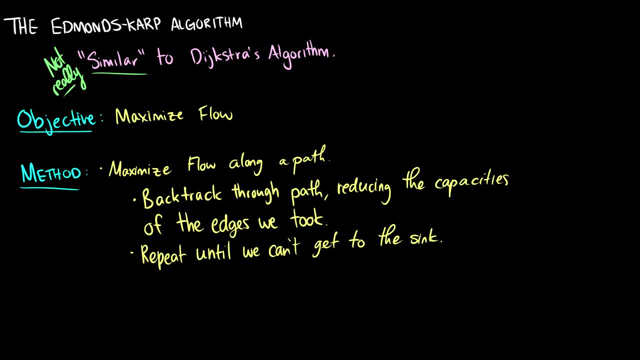 We're going to create a path through our system And we're going to use as much space as we can. Then, once we've got to the end, we're going to backtrack And we're going to say, okay, well, we fit this amount of units through our pipes. 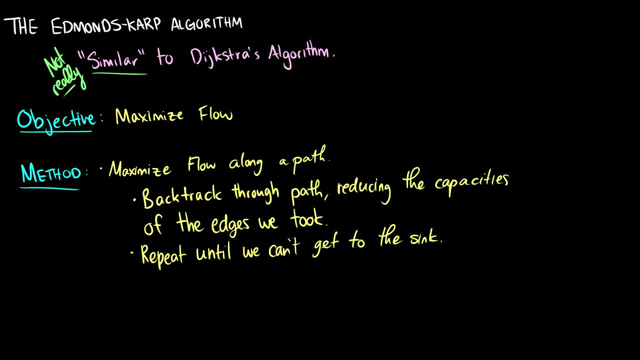 So let's pretend that all of those capacities have been used up And we'll just repeat the cycle until we can no longer get from our source to our sink. So seems a little bit difficult at first. Might be a little bit hard to wrap your mind around. 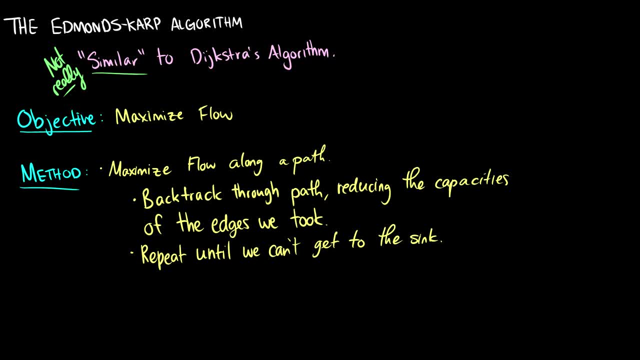 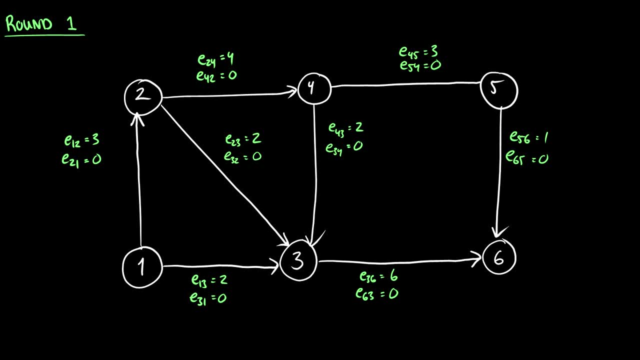 But we'll do the mathematics and we'll do the example. So here is our first round. So this algorithm goes in several rounds. We go through the graph multiple times And you'll see I've sort of changed the notation up. So what I've done here is I've split all of our edges up into two directions. 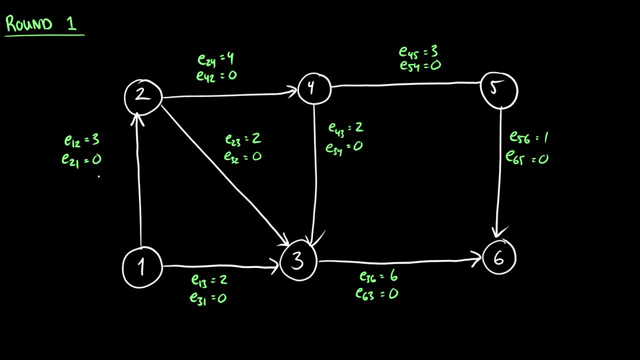 So, for instance, E means the amount of flow we have available from one to two is three And the amount of flow we have going backwards is zero. So I'm going to label this as capacity, And this is going to be what we've used. 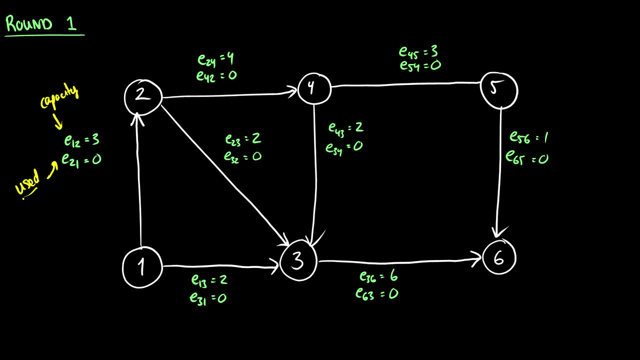 So we've used zero flow out of it. This is like our tracker, because we want to track to see how much we've used every single time. So this screen is going to get a little bit messy, But we'll go by this step by step. 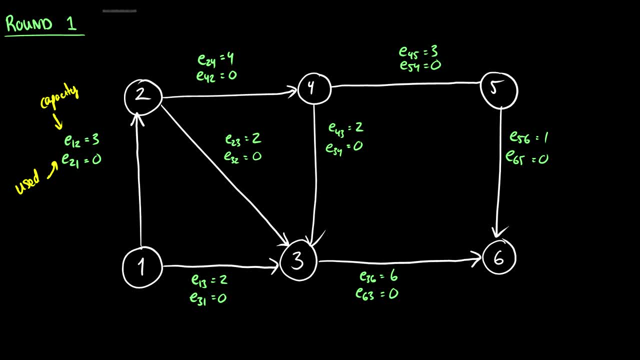 So first we start with our source node And we label it N0 for our first set of nodes, And in this first set we say, okay, where can we get to? And we can get to two, And we can get to three. 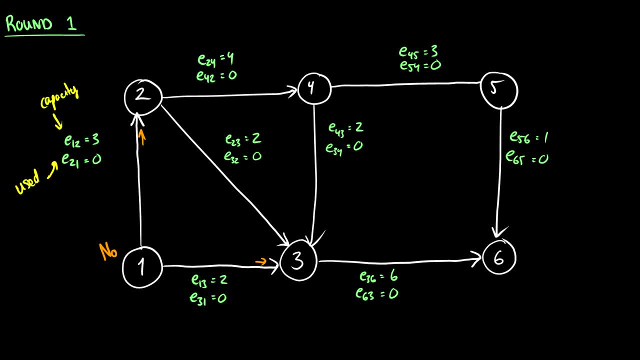 So what we do is we move to one of these nodes. So let's say we move to two And we ask ourselves: okay, how much can we get out of it? Well, we have a capacity of three, So we can get three out of our second node. 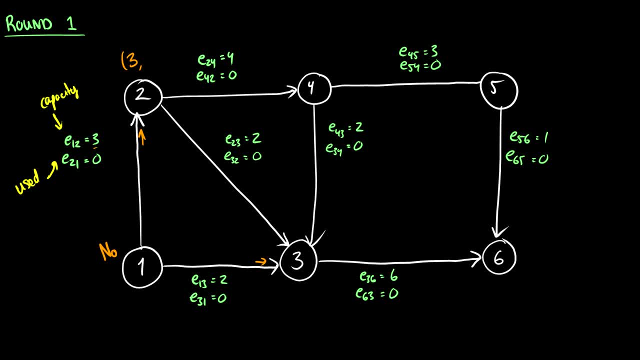 So this first edge from one to two, we can get three out of it. And where does it come from? It comes from the first node, So we label it S31.. And this is the amount of flow. That's the three. 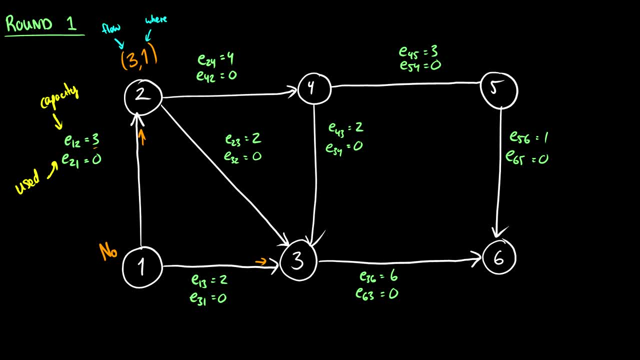 And the one is where we came from. Okay, So where else can we get from the first node? We can get two, three. So how much can we get out of three? Well, let's look at the edge: one, three. 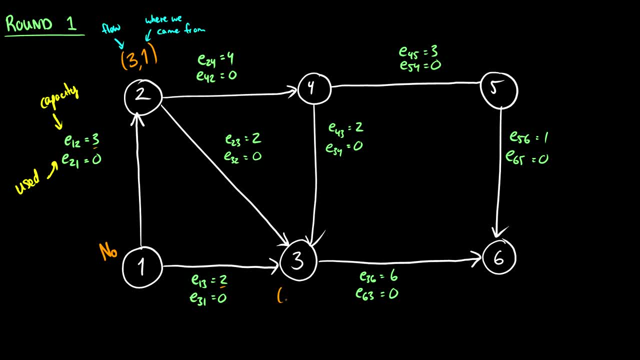 We have two available, So we can write this as okay, we have two available And it's coming from one, Okay. So those are all the nodes that we could reach from one. So now what we're going to do is we're going to say, okay. 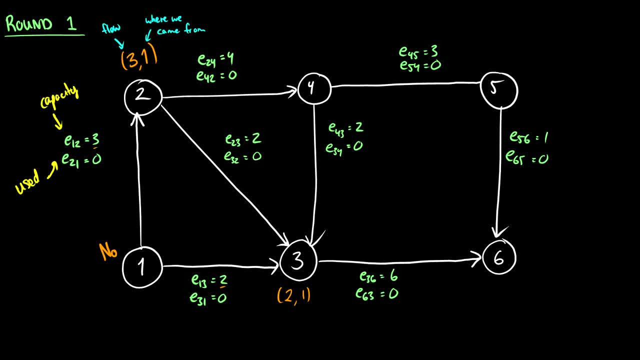 if we could get to a node from N0, we're going to label it as N1.. So this is our N1 set of nodes. It's two and three, So now we'll start with the smallest number, two. So where can two go? 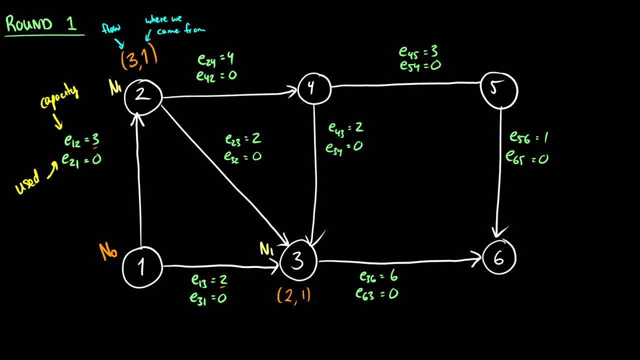 Two can go to four. So from two, how much can we get out of it? Well, we say that we have a capacity of four, So we could get four out of it, But we have only three available at this point, Because we could only get three from one. 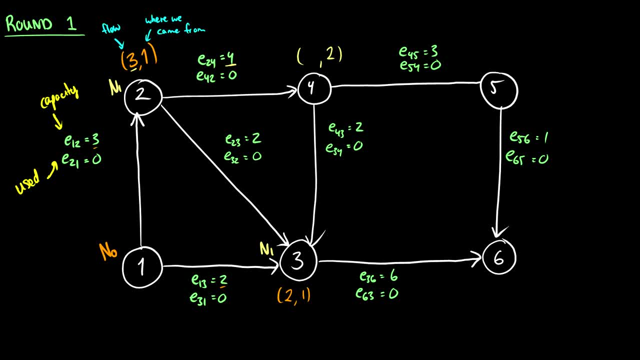 So the most we can get from the edge two to four is three, So we're going to put a three in there. Okay, And can we get two anywhere else? Well, we can get to three, But we can't get to three. 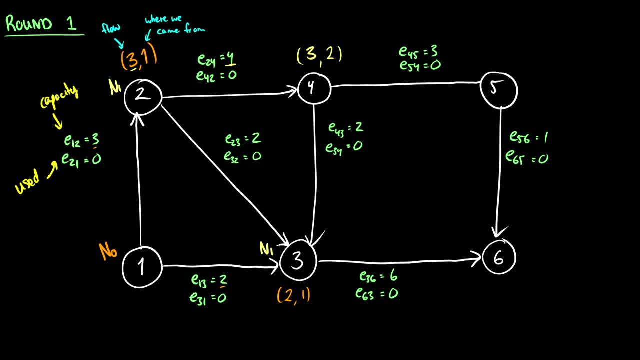 But we've already been to three, So we'll just ignore it. This is a little bit different from Dijkstra's algorithm where we'd say: wait a second. if we can do better, then we're going to replace it. But in this algorithm we're not going to do that because we're looking to 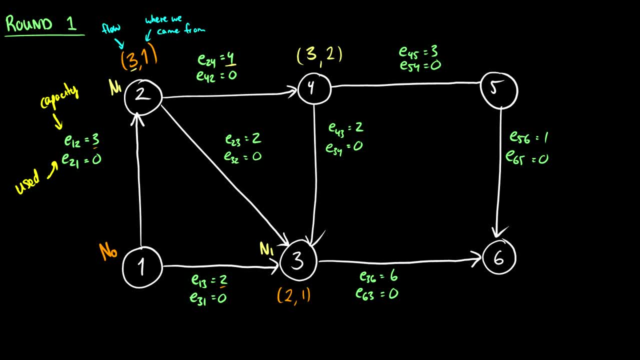 exhaust our pipes. We're not looking to distribute our flow. We're looking to go down a path and say, shove as much as we possibly can into it And then, once that's exhausted, we'll go try another route and we'll keep shoving water as much as we possibly can through these pipes. 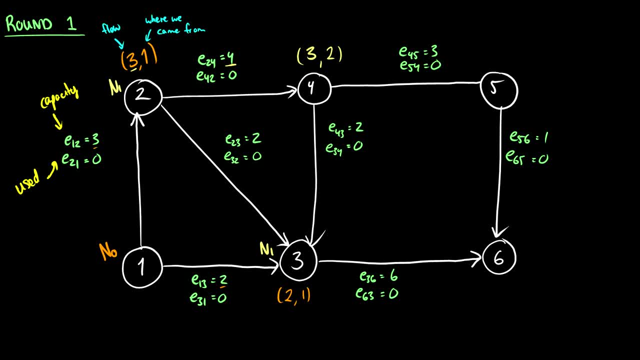 So we're not going to go over this old node. So now we've done two, Let's move on to three. So where can three go that nowhere else has been? Well, it can get to six. It can get to our sink node. 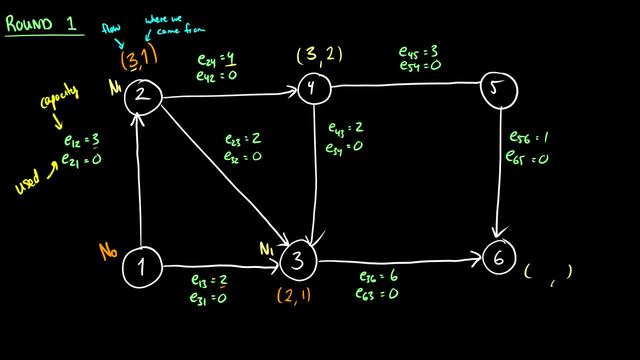 So it comes from three. And how much can we get out of it? We can get up to six, but we only have two, So we can get two. Okay, So it is done when the sink node is labeled. So I know you're saying: hold on a second. 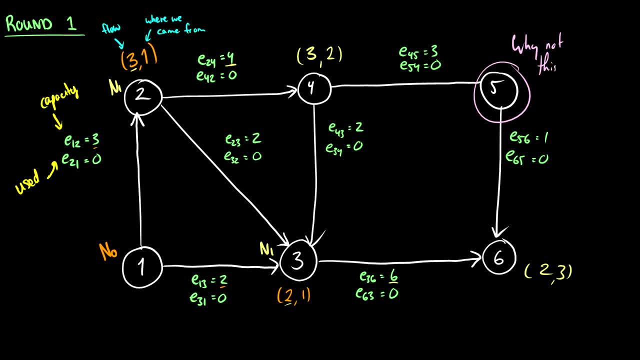 Why not this guy? And the answer is well, we'll deal with him later, But for now we've gotten to our sink node, So we'll do the backtracking step. So what does this graph tell us so far? Well, we have a path here from six. 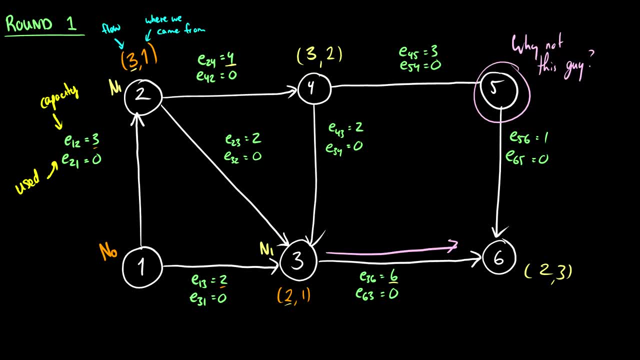 We went from three because we got two from three. From three we got two from the first node. So we have this path right here And this is the path we took. So we got two out of this whole path. We got two units of whatever we're pushing through out of this path: one, three and six. 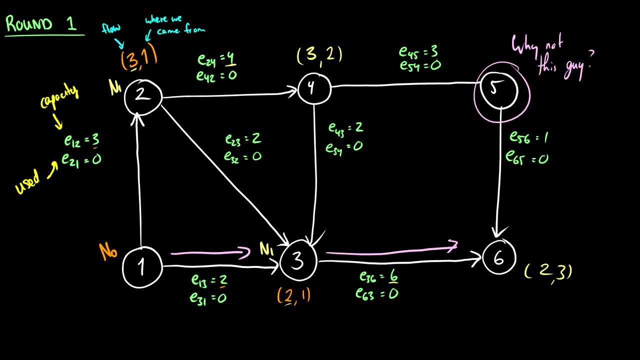 So what we'll do is we'll say, okay, let's pretend from now on that we have two units of water already rushing through here, So we're just going to pretend it's always used up and not consider it for the next cycles. 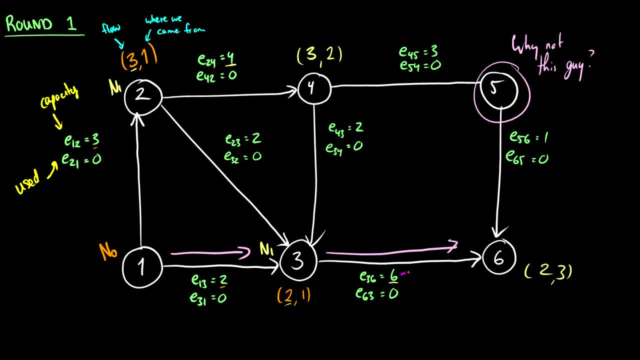 So what we do is we subtract two from all of the edges we've used, And then we're going to add two for how much we've used. So this is just our mental track here. So for one- three, we have zero space left. 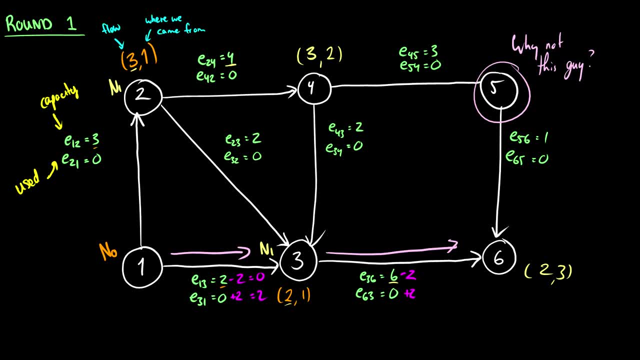 And we've used two space And, for our edge, three, six. we have a total of six available, but we've already used two of them, So we'll just have four remaining, And now we've used two. So this was the first round. 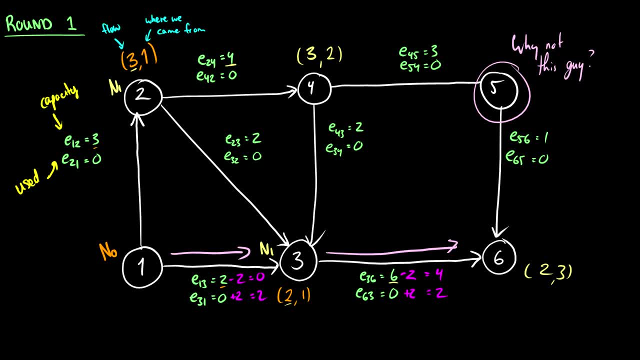 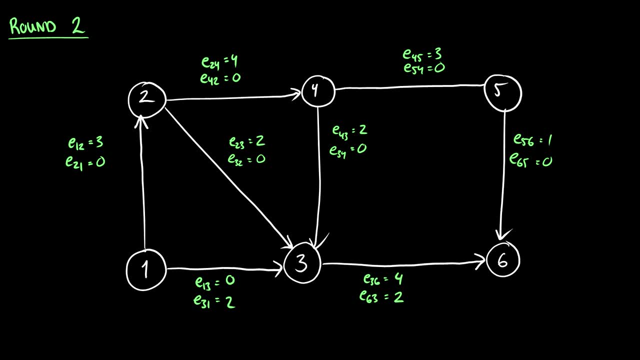 We have now updated our edges, We've backtracked through And we've reserved our flow, So now we just start over again. So, as you can see here, I've updated our flow, I've updated the numbers. I just cleaned it up a bit by making these slides in advance. 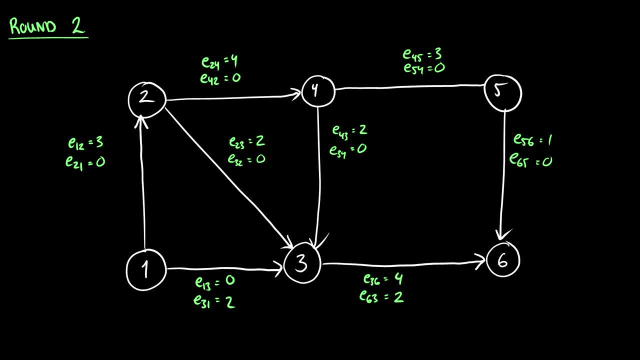 So now, when we consider things, we start back at the source node and we try to get back to the sink So we can do the same thing. Okay, from one to two, we can get three out of it, and it comes from one. 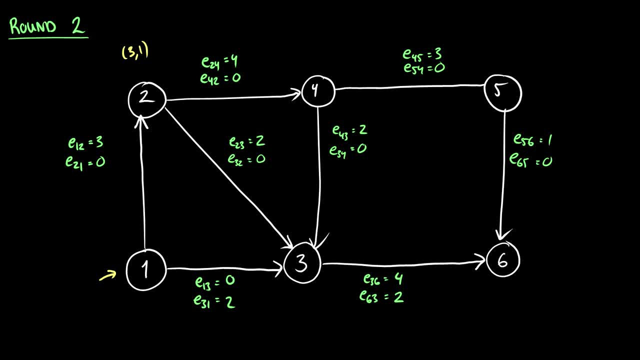 But what about this case now? What about one to three? Well, we can't get to three anymore because there's no capacity left. So we just leave it as blank and we say: okay, we can't get to three from one, so let's just not label it. 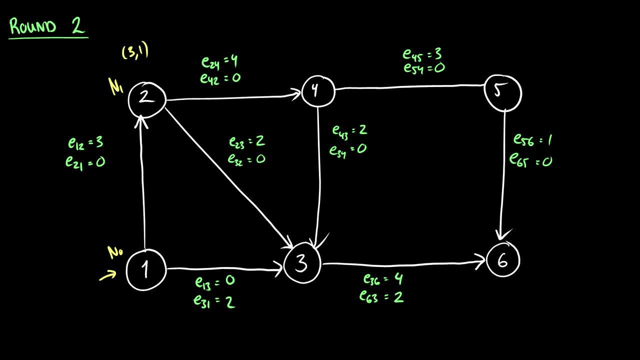 So again, this is our N0.. So now this becomes our N1 here. So where does two go? Well, two goes to four. So, just like before, we have a capacity of four here, but we can only get three out of it. 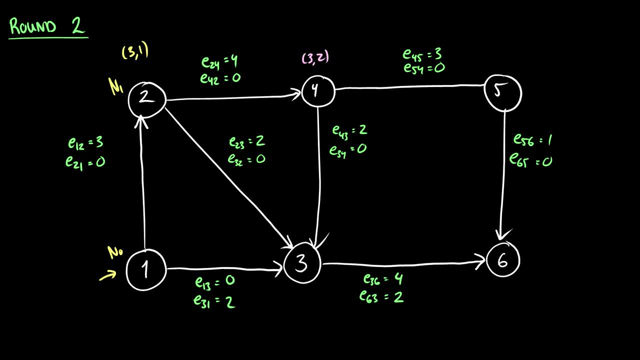 So the most we can get is three, and that comes from two. So when we take a look at three here, we can get to three from two. And how much can we get out of it? Well, it has a capacity of two here, so we can get two out of it from two. 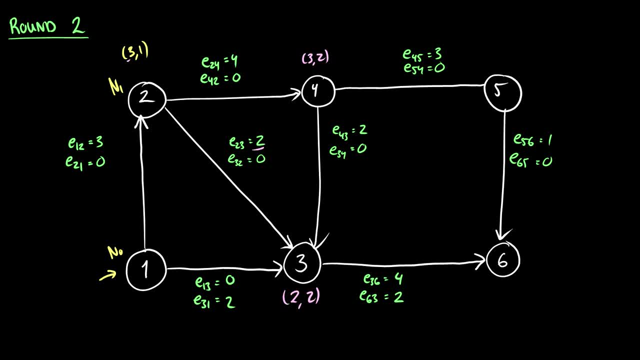 Because we have three already, but we can't fit more than three through the pipe. we can only fit two. So we can say, okay, the most we can get from this edge, two to three, is just two. So that's all two could reach. 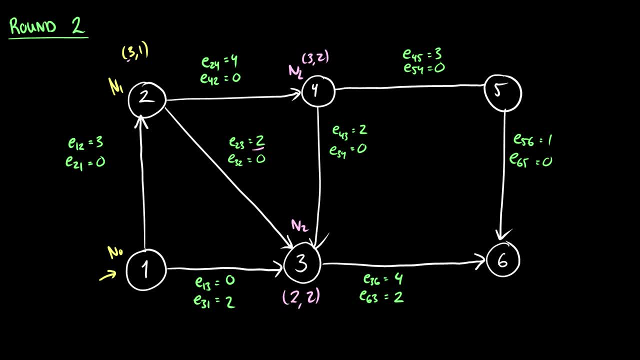 So now these are our N2s. Okay, so again we start with our lowest number and let's see where we can go. Three goes to six. It has two right now. It has a capacity of four between three and six, so we can get two out of it and it comes from three. 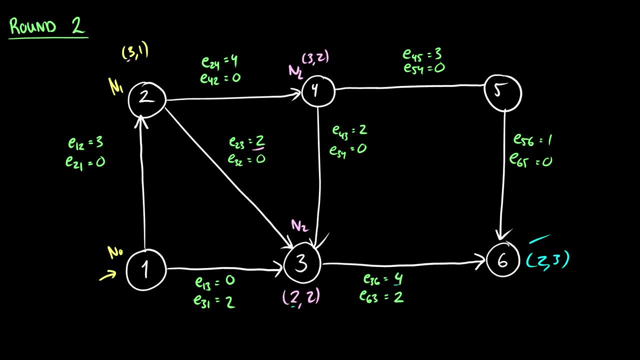 And now our sink has been labeled. so we are done. So let's backtrack. Where do we come from? Well, we got two from three, and then we got two from two, and then we got three from one. Okay, but as you can see here, we had to ditch all three. 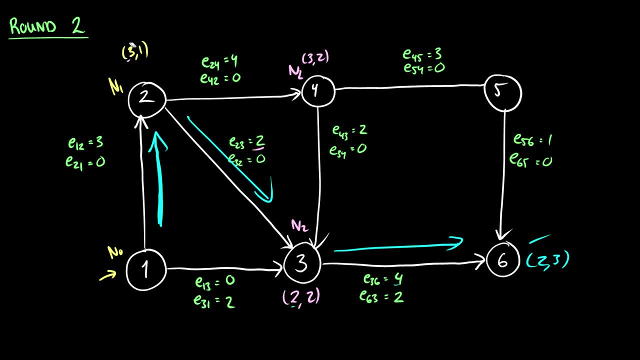 We had to just take two, But really what matters is that we take the minimum amount. So here we can see: we got two in our three to six, We got two from our two to three. So we're just going to subtract two from all of our flows. 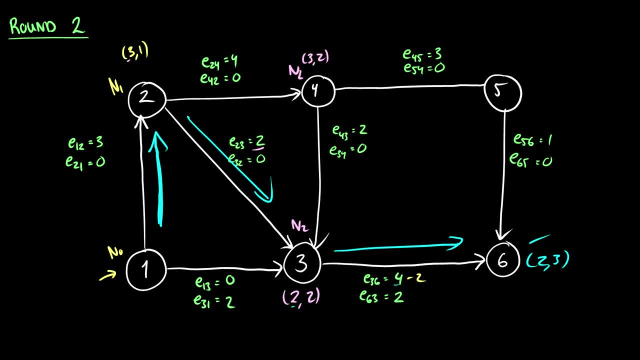 So this had a capacity of four, but now we're using two more of it, So it ends up as two and we've used two more, So now it's two plus two is four. So that's saying we used four out of the six capacity for this three six edge. 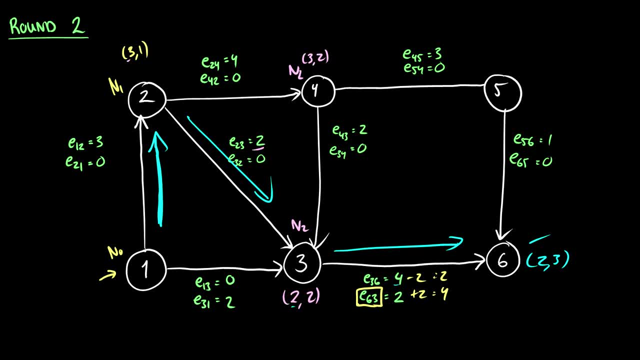 Then we went from two to three and we took two from it. So now there's no more capacity available in this two to three node. So that's zero and two, And we use two from one to two. So, yeah, So, even though we have three written up here, 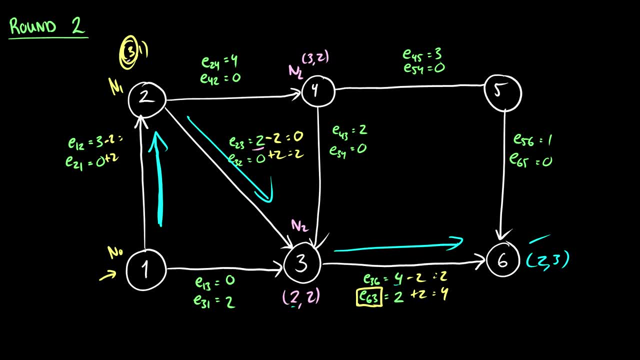 we didn't use all three, We just used two of it because only two made it to the sync node. So we just subtract two from our first and we add two to say, okay, well, we've used two here. So that was the second round. 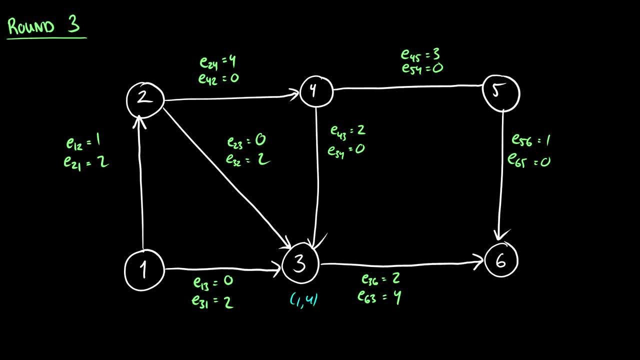 So now, when we update our numbers here, this is what we have left. So, as you can see here, we only have two remaining from our edge from three to six, and we only have one remaining from our edge one to two. So this should be the final bout because, as you can see here, 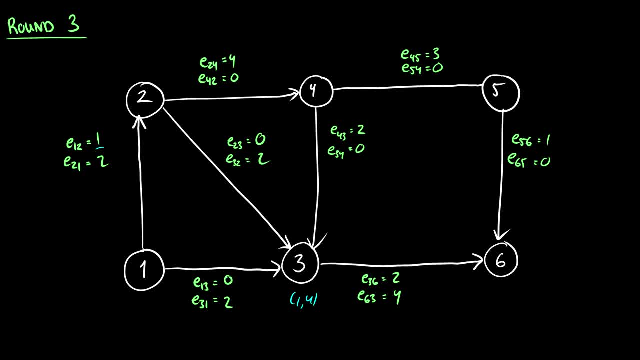 we only have one capacity remaining and zero capacity remaining for our one to three edge. So let's see what we can do. We start with our source node, We move up to number two and we say, okay, we can get one unit from the first node. 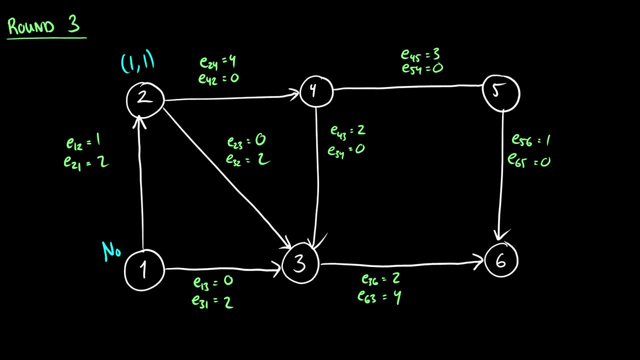 And that's it. So we can't get to this third node here from one. Okay, So what about from two? Well, from two we can go to four. We can get one out of it. It has a capacity of four, but we only have one flow we can use. 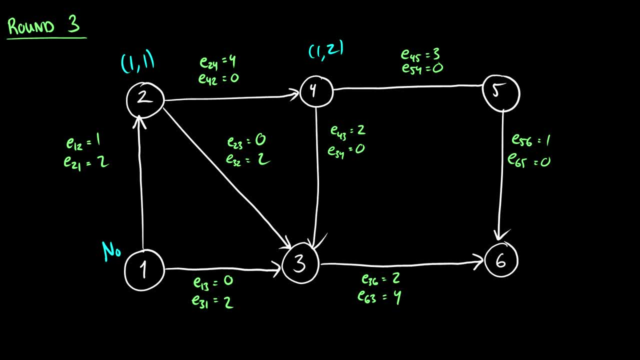 So we can get one out of it, and it comes from two. What about to three? Well, we can't go to three anymore, because this has no capacity. These two lines are now cut off, So we can't go that way. 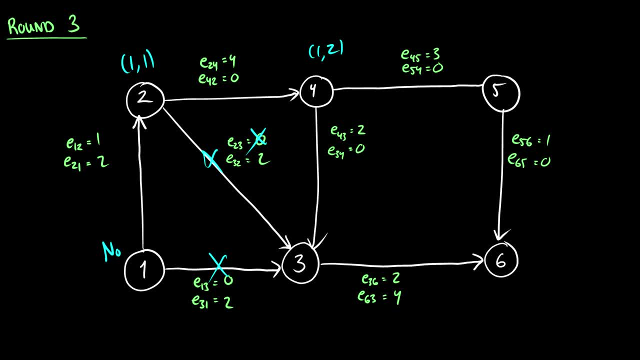 We can only go to four. What about now? So we go from four. Well, we can go from four to three, because there's two capacity here. So we can say: okay, I can get one unit from four And then from five, I can also go there. 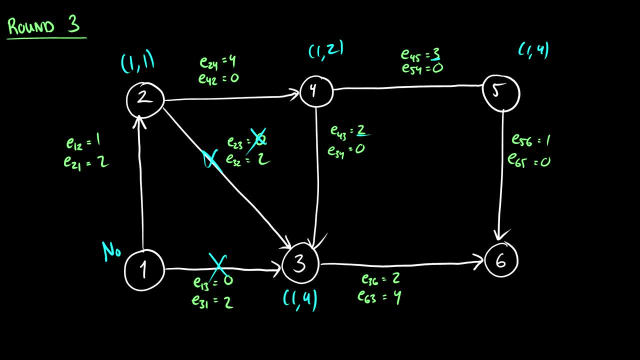 So I can get one unit from four and I can go to five because we have a capacity of three. Okay, So now you could go from five to six or three to six, But if you remember the algorithm, we always use the lowest number. 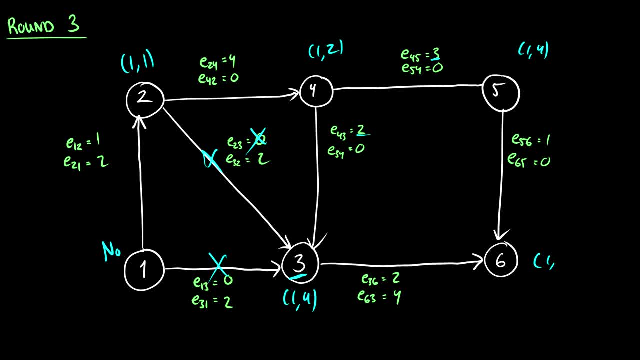 So we're going to go from three to six and we can get one out of it because it still has capacity of two, And that comes from three. So we've labeled the sink node. So now we are done. So let's backtrack and update some of our numbers here. 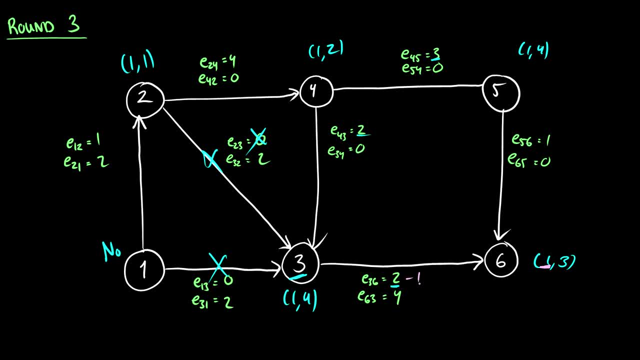 So we've got a total of one flow from three. So that's minus one plus one. So we now have one capacity remaining in our three six edge and we've used five. We've got one from four. So we should subtract one and add one here. 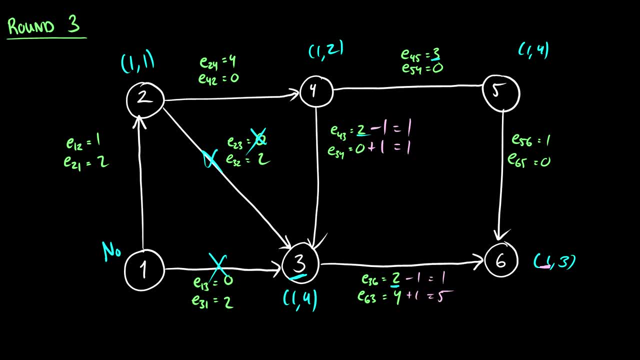 So that means that we now only have one capacity remaining from this fourth three edge, and we've used one. We got one from two. So this thing that had four capacity here now only has three and we've used one. And of course I accidentally erased that line. 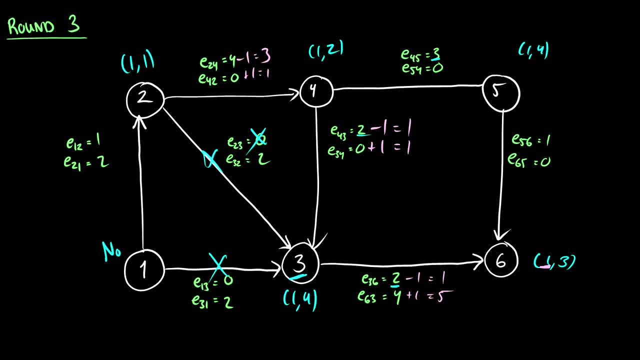 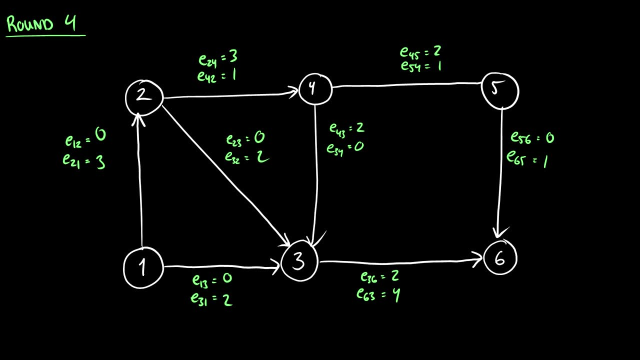 Okay, And now from two we get one flow from one. So now we have exhausted our one two edge. Okay. So let's update some numbers here. Did I miss add That should be three. So two plus one is three. 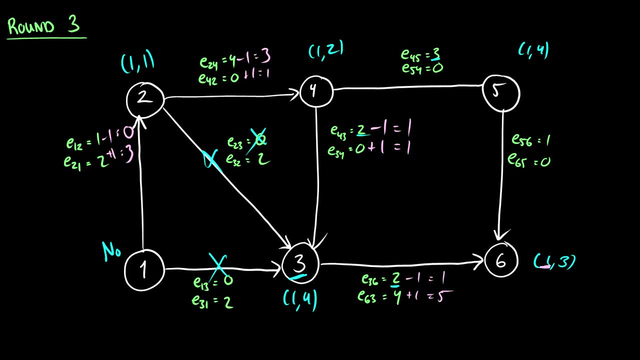 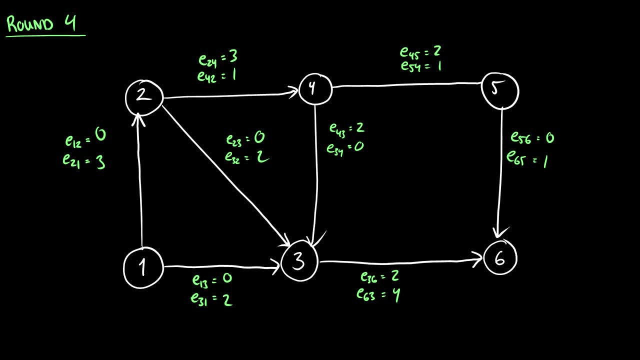 Okay, I can add. I'm good at math, sometimes I pretend I am Okay. So round four: We know we're done when we can no longer reach the sink node from the source. So can we go from one to six? 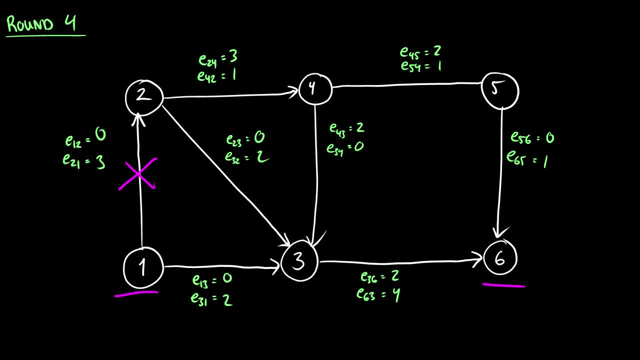 Well, we can't go to two because there's no capacity left, and we can't go to three because there's no capacity left. So we are done. These are the final numbers. So you're saying, okay, well, how do I draw a flow graph from this? 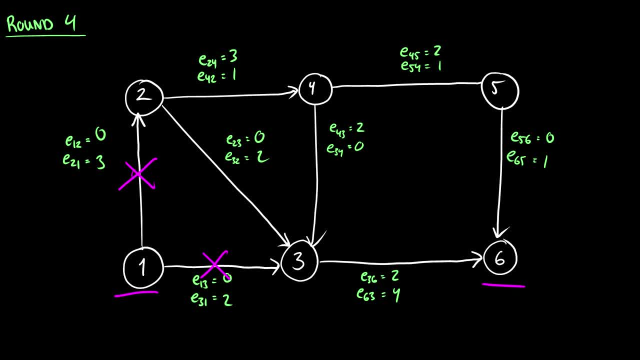 Well, if you remember from before, we label our edges with capacities and flows. So what I'm going to do first is I'm going to label all the edges with how much flow we've used. So we have a three flow from one to two. 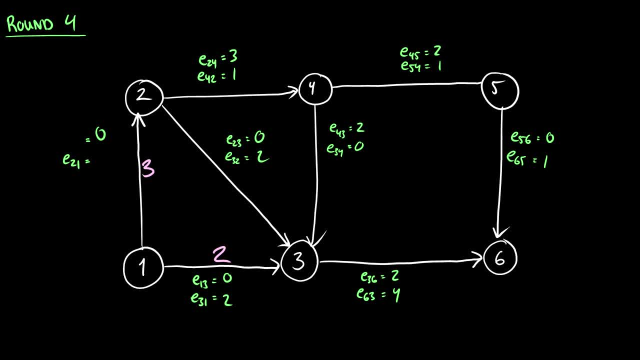 We have a two flow from one to three. Again, I'm just looking at these numbers at the bottom here. So these are how much we used. If we take a look at these numbers that I'm circling So we can label these edges. 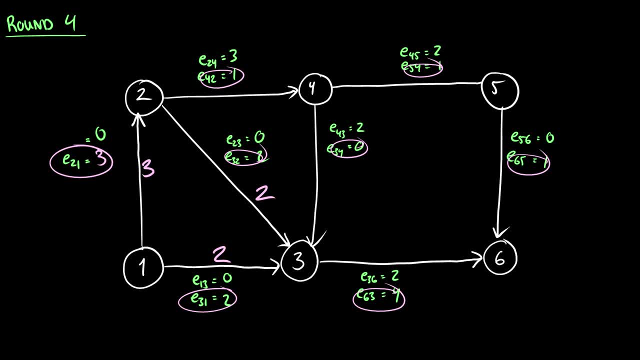 So that's three, two. Two to three is using two, Two to four is using one, Four to five is using one, Five to six is using one, Four to three is using zero, And three to six is using four. I just realized now that in this example, 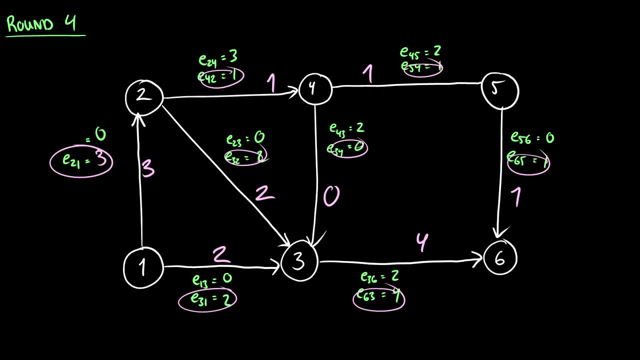 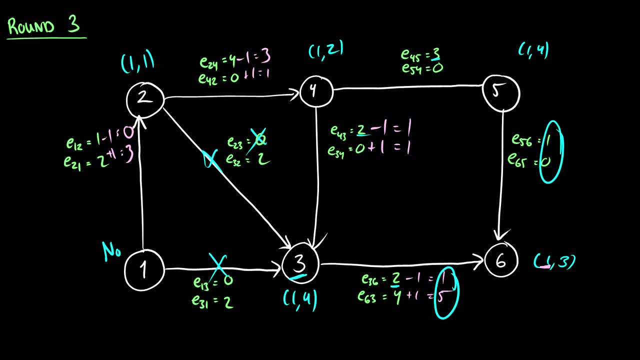 I went from five to six instead of three to six. So, as you can see here my numbers, they are a little bit off, But it does not matter which one you use, as long as you pick one For this demonstration. I just picked the lowest number. 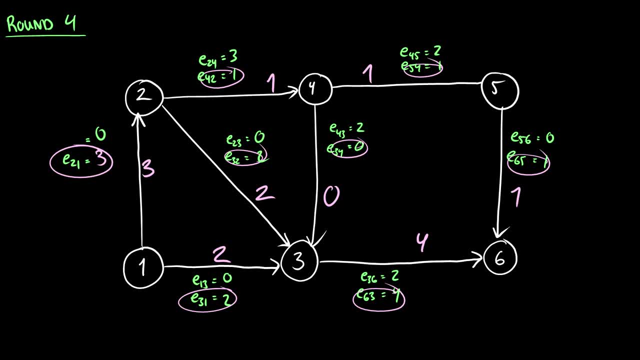 but I guess when I made the slides earlier I used five instead, So either way works. We'll just say that we use the flow from five to six, But what we could do is we could change these numbers if we want Five, zero. 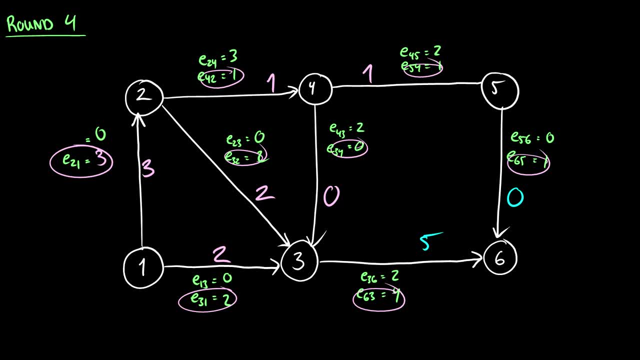 And they would be the same thing, because that's how I did it in the example. But for the sake of this, let's just update it and say it's four one, But they are the same. Okay, so that is our flow. 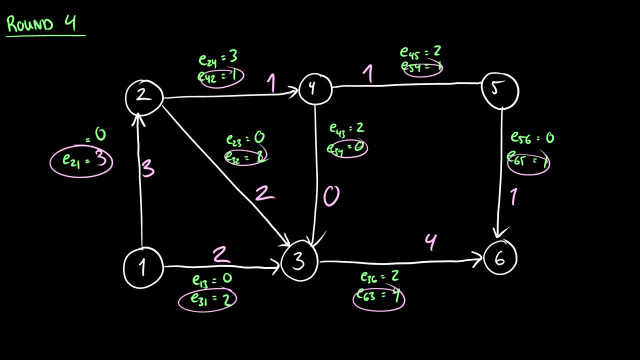 So this is pretty much done. You could say this is the flow between the networks. Let's check our things here: We have five leaving the source And we have five entering the sink. So we're good, We have a source, We have a sink. 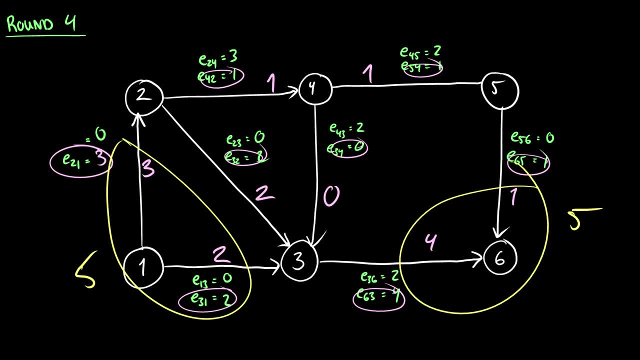 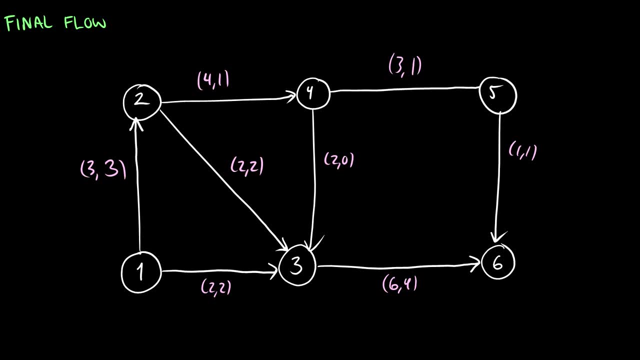 And the out degree of the source is equal to the in degree of the sink. Therefore our flow network must be good. So we can summarize this And we can put this in its capacity flow form. So, as you can see here- the first one- it has a three capacity. 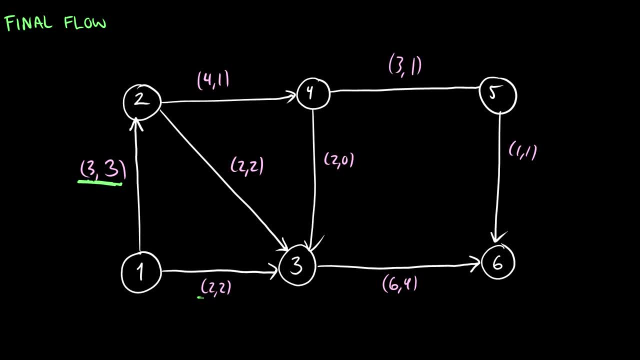 And it's using all of its flow. Our one to three edge has two capacities using all of its flow And this three to six is using four out of its six available. Five to six is using one out of one. Four to five is using one out of three. 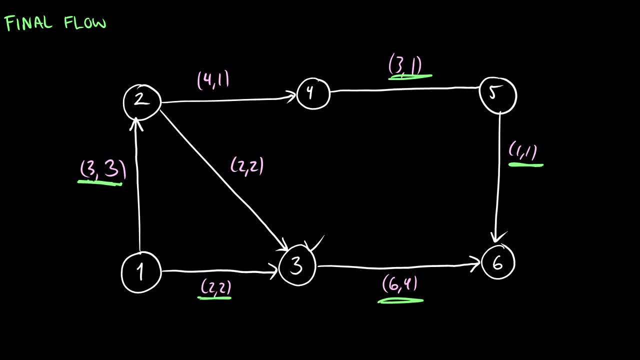 Four to three is using nothing, So why do we even have this? Let's forget about that. Two to three is using all two of it, And two to four is using one out of the four available, So we can even check each edge. 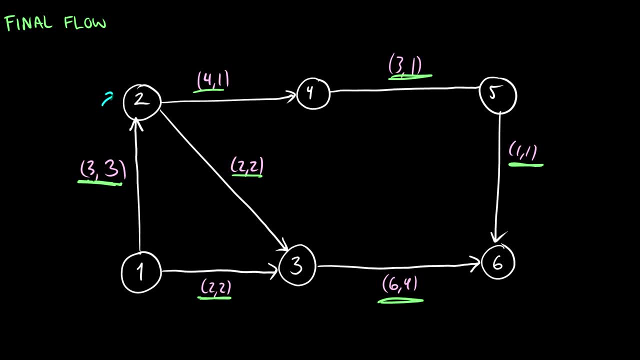 And we can say: okay, well, there's three going into it, So there must be three going out of it. So there's one going out there And there's two going out there, So we're good, One going into here.